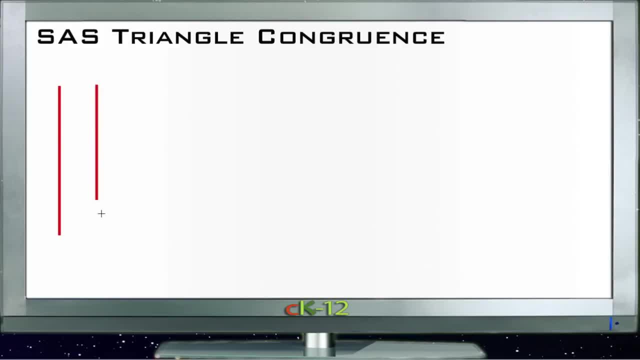 sort of a medium length one here and ask you to build two triangles out of them. you could build pretty much any number of triangles. I mean, you could make one that was sort of straight across with the other side and you could make one that was sort of straight across with the other side. 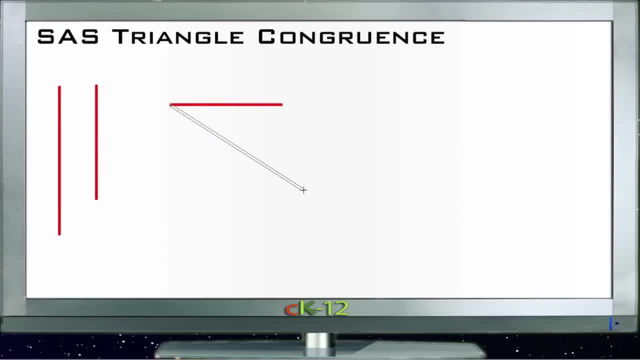 You could have the medium length one and then way down this way with the longer one, and then you'd have another side that was just a little bit shorter than your medium length one, maybe over here. Or you could take your medium length one off in this direction and your long one off in this. 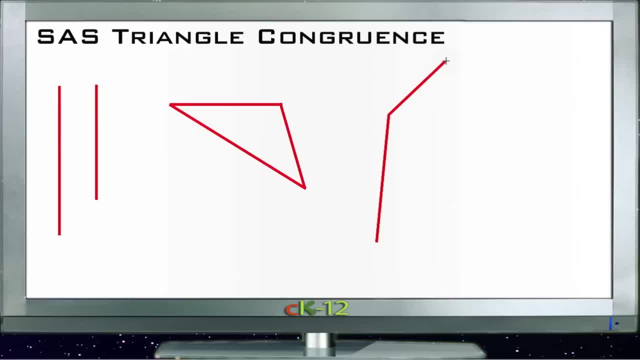 direction and that would make your missing side really long, coming clear down from up here. So you can see that just by knowing two sides we can't really say anything about a triangle. However, if I took those two sides and I took the long one, and I took the long one and I took the, 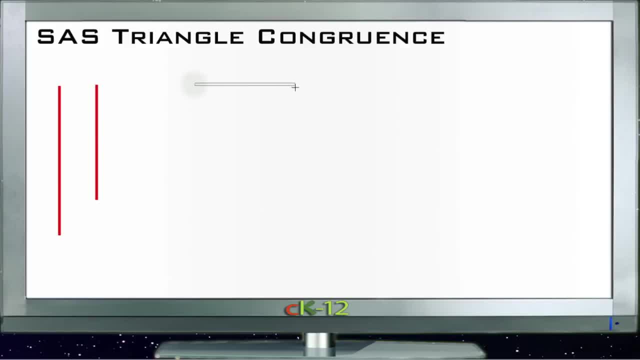 sides that I gave you originally, and I didn't just tell you that you could use those lengths, but I also told you that the angle between those two sides was fixed. Let's say it had to be whatever. this angle- we'll call it 45 here- had to be this specific 45 degree angle, right here, With that 45. 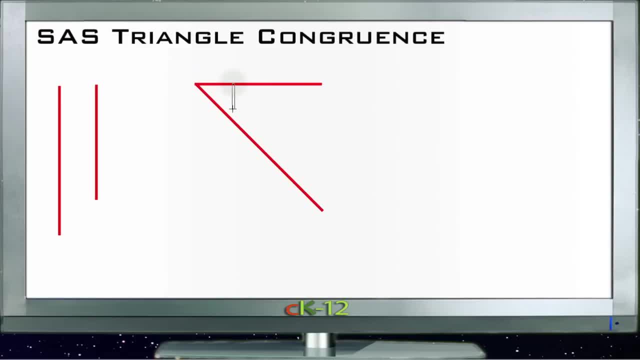 degree angle fixed in place here. whoops here. now the number of triangles you can make out of those two lines is drastically reduced. In fact, it's reduced right on down to one. There's only one way we can connect a line. 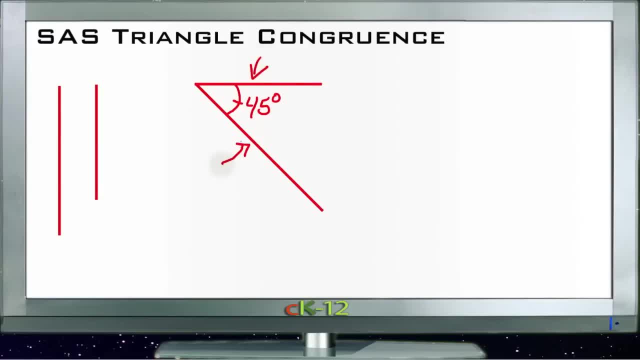 that's this specific length and this specific length that are sort of anchored in place at this 45 degree angle. The only way to connect those two is with a line that goes from here to here. There's no other way to do it. You can't connect these two lines with any other length of line. 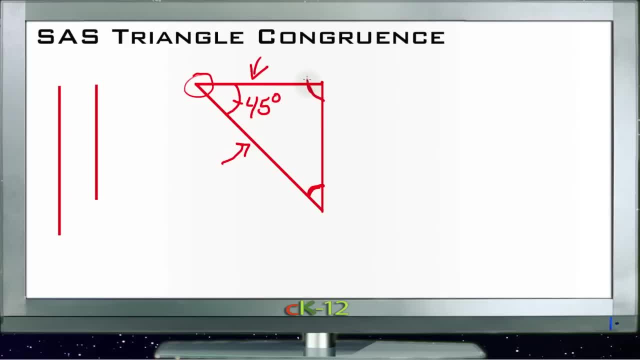 or any other different angle than the two that appear right here. So once you have those lengths and the angle in between them fixed, the triangle itself becomes fixed. So side-angle-side triangle congruence is pretty slick. It doesn't take a whole lot of information, but it allows us to show. 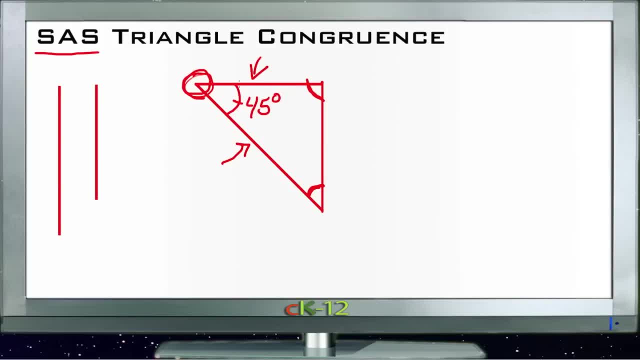 right away that two triangles are the same if the two sides and the angle in between them match. Let's take a look at the example problems and see how this works.